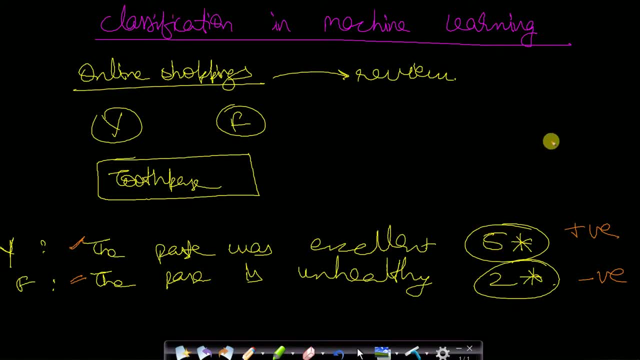 review and the stars it can say whether it's a positive review or a negative review. So you need a model. Okay, so what you need is a model on feeding which, if you feed a review to this model, it will say whether it is a positive review or it is a negative review. And if you assign this, 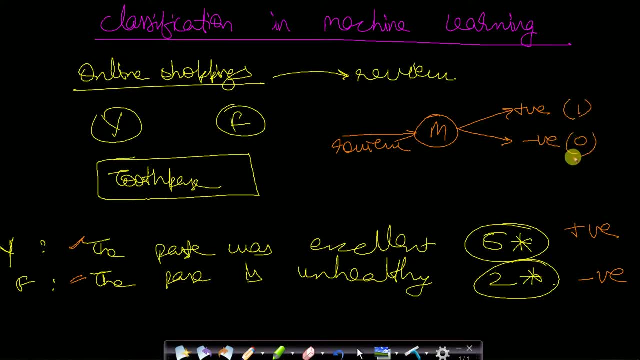 positive review to be class one, then this negative review can be taken to be class zero. And since this review can either be a positive or a negative review, it can be a positive review or it can be negative review, So a single review belongs to maximum of two classes. 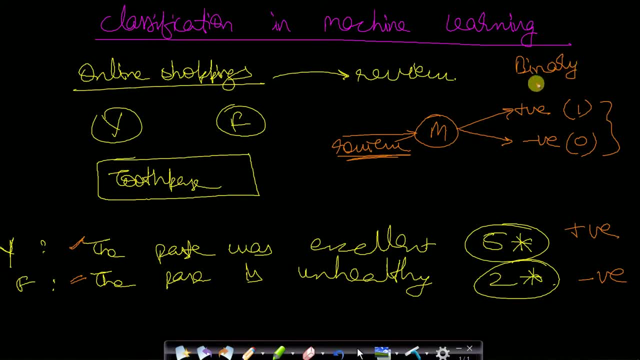 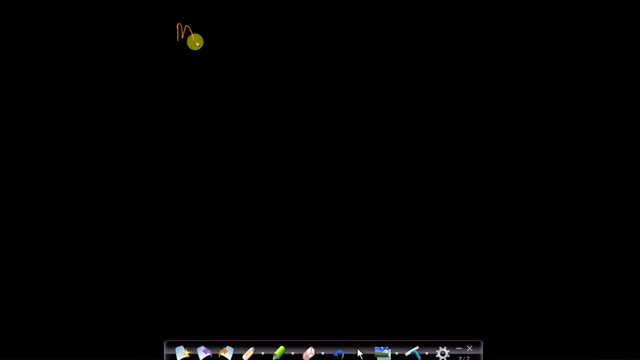 And so this is known as a binary classification problem. Okay, binary classification because we can differentiate this given review into two number of classes, Either to be a positive review or to be a negative review. Okay, so let us first understand what is binary classification and how does it work? by using a model. You need something known as a model. 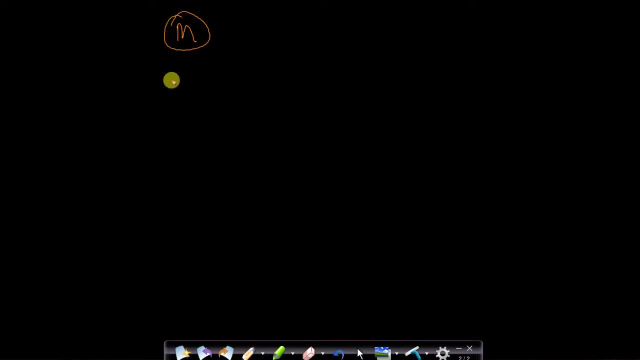 Okay, so how your model can differentiate between a given review, whether it's a positive or negative? You need to train the model, Okay, so how will this training be done? If you are given a model, then you will have to feed it millions of reviews, Okay, 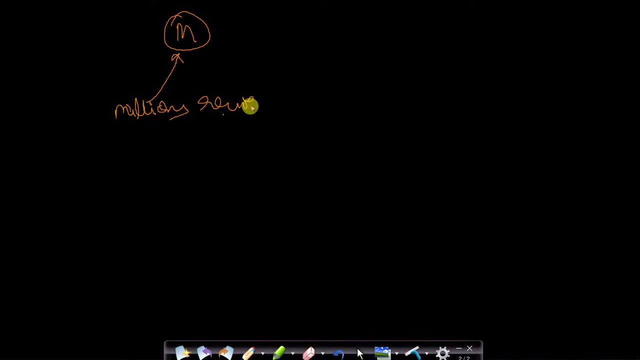 you will have to feed it millions of reviews And this will be included along with the class labels. And what will be the class labels here? The class labels will be: either it is a positive review or a negative review, So there will be a. 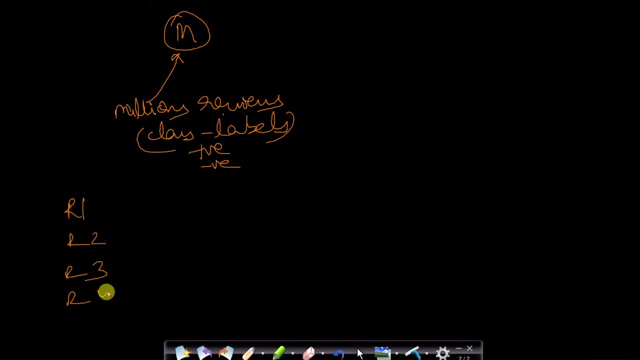 let us say: review one review, to review three, review four and so on to review n- okay, And then you will have either it's a positive or a negative review, a positive or a negative review, and negative a positive, and so on. let us say the last one is a negative review. okay, now you are feeding the review along with the 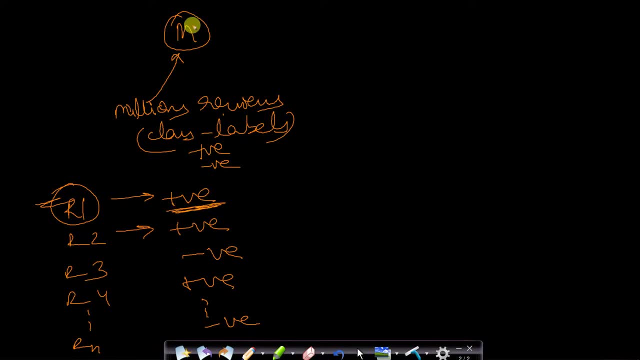 answers whether it is a positive or a negative review, and what will this model do? this model will understand that this review means a positive review, this review means a negative review- okay- and it will also see the stars. let us say that stars greater than equals to three means a positive. 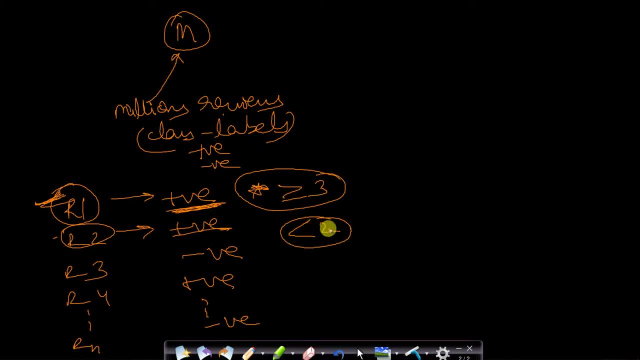 review and stars less than two is a negative review. less than equals to two is a negative review. okay. so this is a very, very simple model. if i draw a two-dimensional figure of this, then if i assume the green points to be my positive reviews, like this one, okay, and then i mark the. 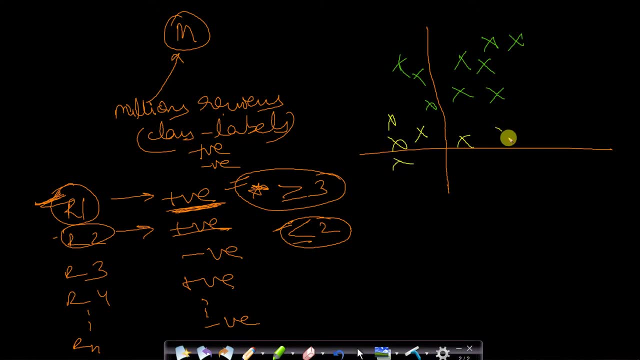 yellow points to be the negative review. okay, so these are all my negative reviews. then how will this model understand, given a review, whether it's a positive or a negative review? this model will draw something known as a decision boundary. okay, so it will mark a boundary which will separate the positive reviews from the negative reviews. okay. 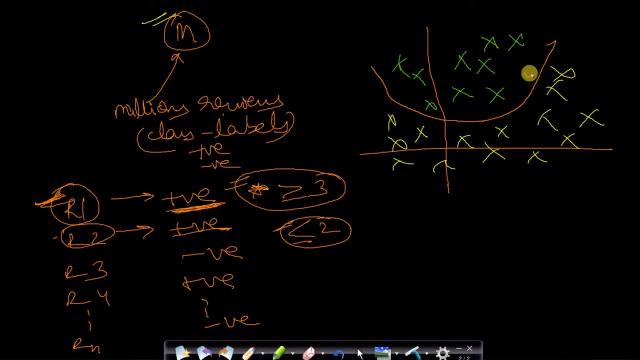 and if you're given query point, let us say this is our given query point. okay, this is our xq given query point. if it falls on on in this region, in the green region, then your model will say that xq is a positive review. okay, so xq. 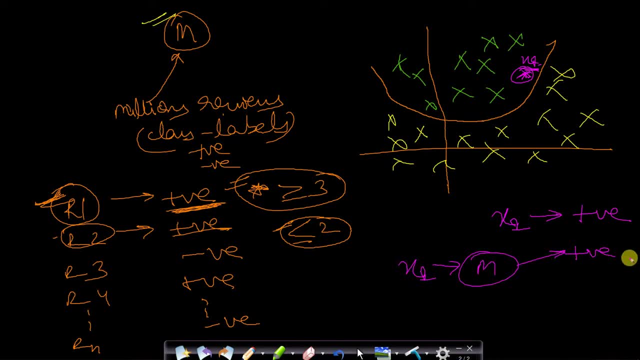 will be fed to your model and your model will say that it is a positive review and it will return class one. if another point- xq dash- falls in this region, then it will quickly say that xq dash is a negative review. okay, so this is how your model can classify given a review. so this is a simple binary. 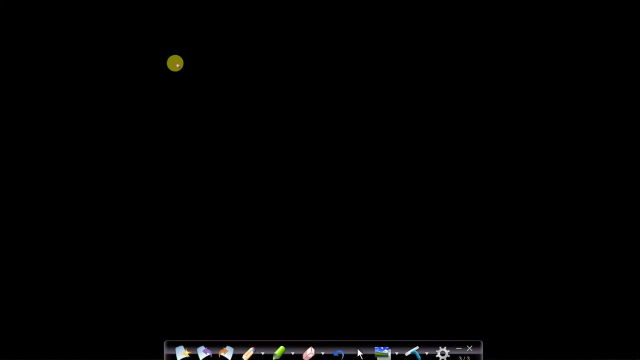 classification example: you can also have multi-class classification. let us take an example of a picture. okay, so this is a picture and you are asked to say what animal it is. then it may be a monkey, a cat, a dog and so on. it can also be an elephant, okay, so there are many classes to which. 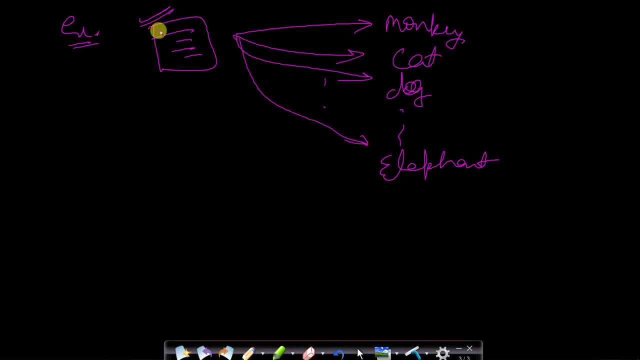 a single photo, the animal present in the single photo can belong. so if you assign a class to monkey, let us say zero. to cat, it's one. to dog, it's two and so on. to elephant, let's say it's n, then you have a total of n plus one classes here. okay, so this n plus one is obviously greater than. 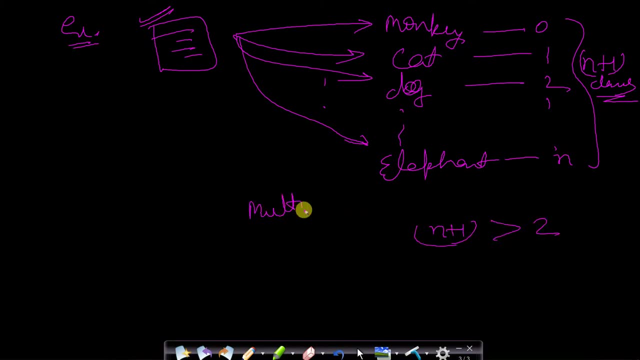 two, and so this type of classification is known as multi-class classification. generally, multi means more than one, but in machine learning generally we use multi for any value which is greater than two, because for two we use the name binary. okay, these two works in the same way. you have a model and you will have to train the model with lots.